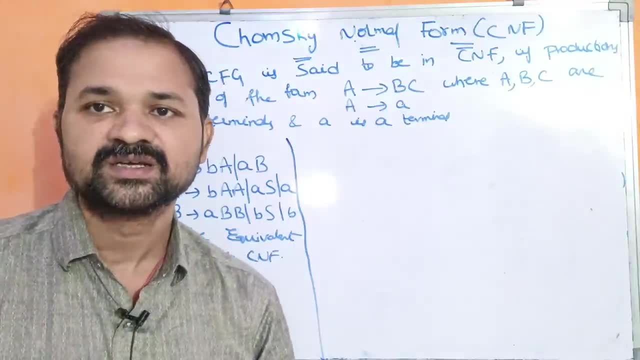 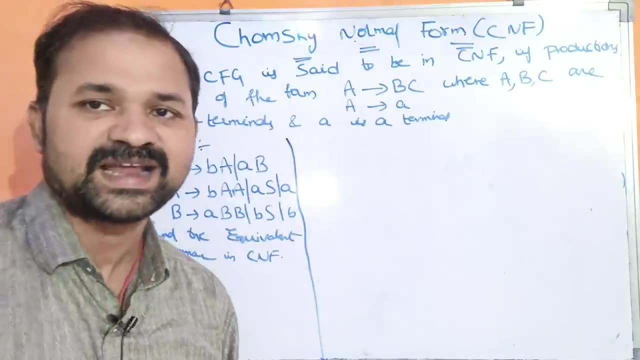 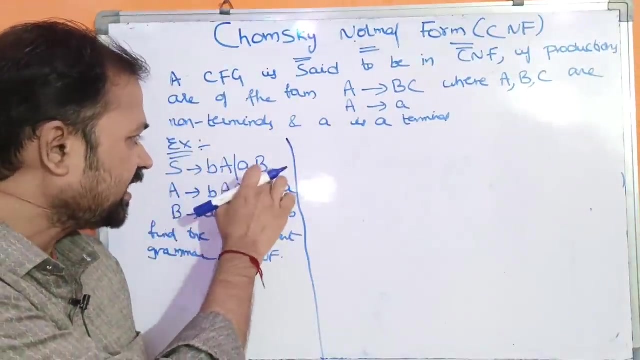 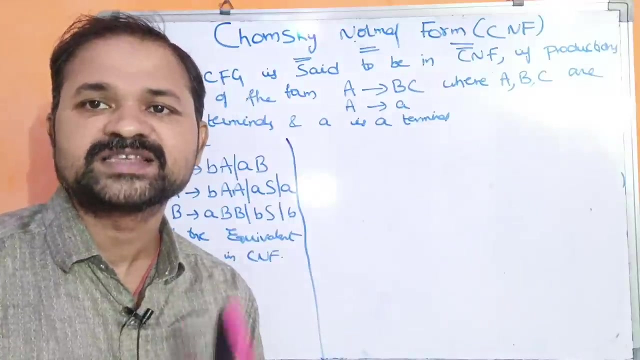 one is by eliminating epsilon productions. Third one is by eliminating unit productions. When we do that, we know that we areೂ. When we do that, we know that we have하게. In conclusion, there are no two ancient 난 of WHAT need and need, nor products. 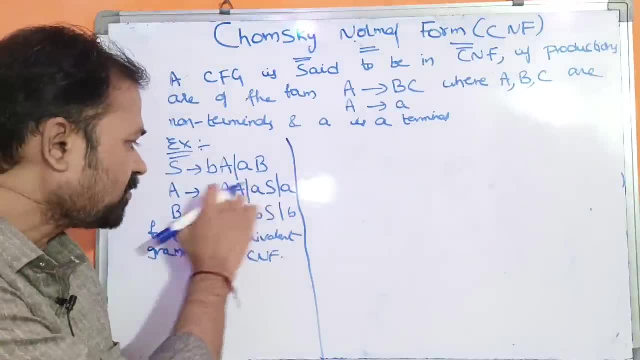 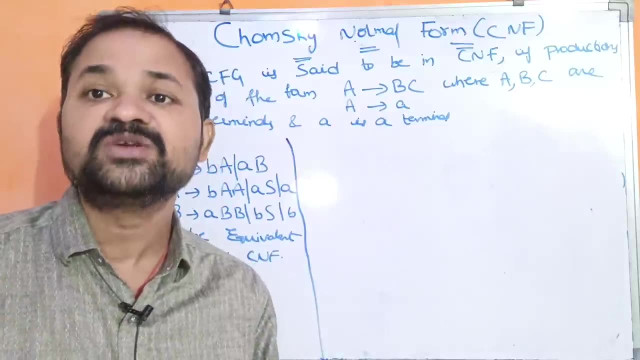 We do not have this einges for이를, the stereotypical question about product culture. we say new thing: Xi, Monum et al. one Find the equivalent word of simpleA Pro entirety days, other nonsnore, OK, Well, that is it. 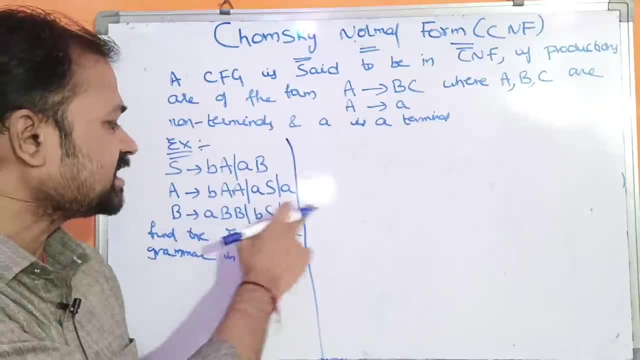 Thank you very much. There were some others of today's guest. See you guys next weekında-s. I will talk to you next week. one non-terminal, But in the right hand side we do not have a single non-terminal, So 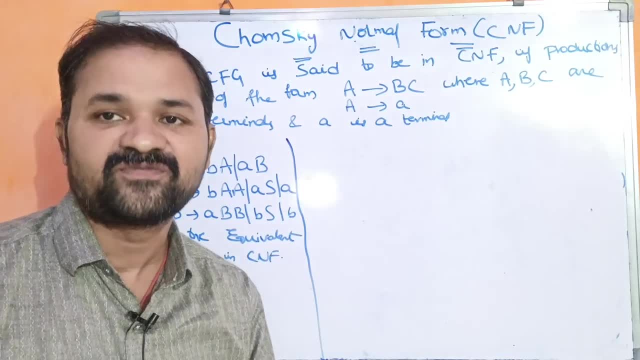 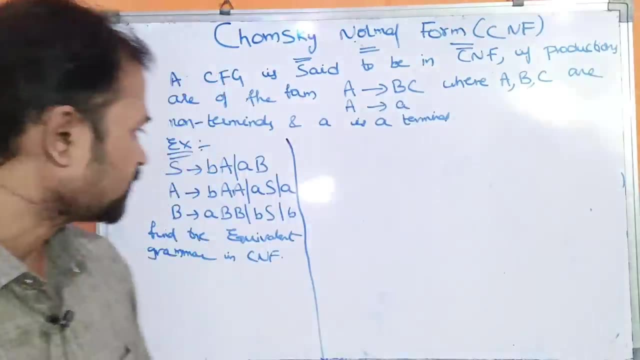 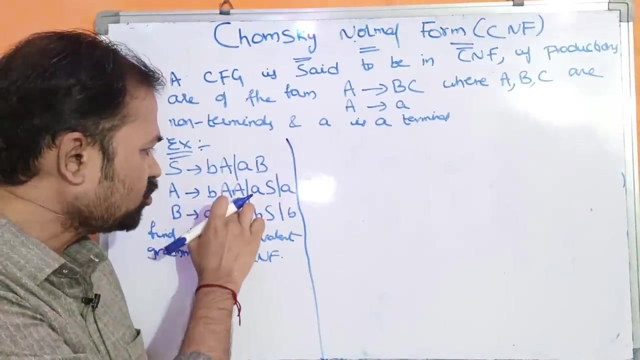 we can say that all these projections are in simplified form. So first observe the projections which are in Chomsky normal form. So if you observe this projection, here we have one terminal non-terminal, one terminal non-terminal, one terminal, two non-terminals. 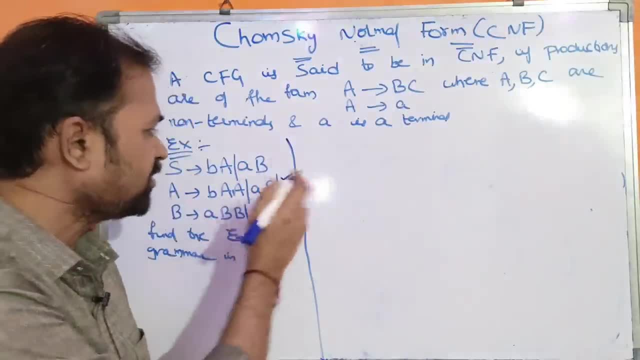 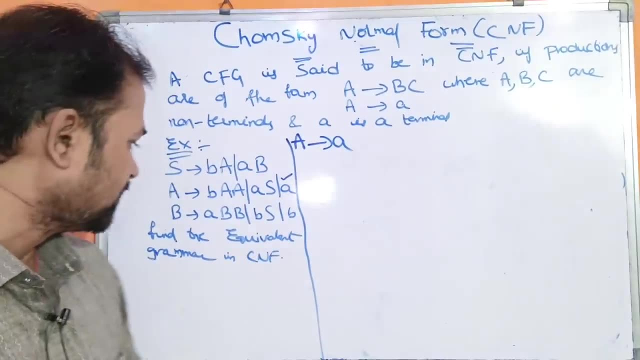 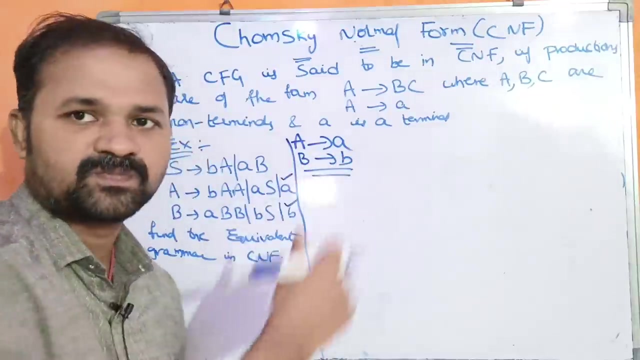 one terminal, one non-terminal. If you observe this, one A produces A, So this is in Chomsky normal form. Non-terminal produces terminal symbol. If you observe this, one B produces B, So these two projections are in Chomsky normal form. So next, what we have to do is: 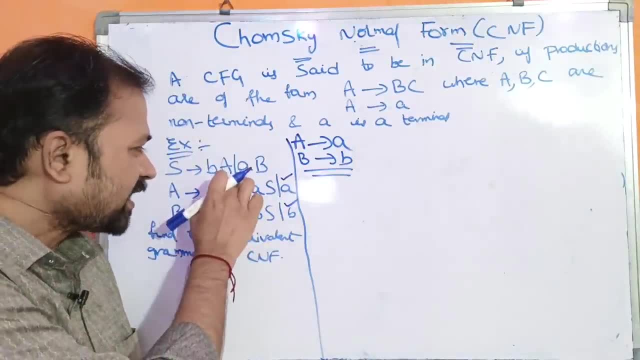 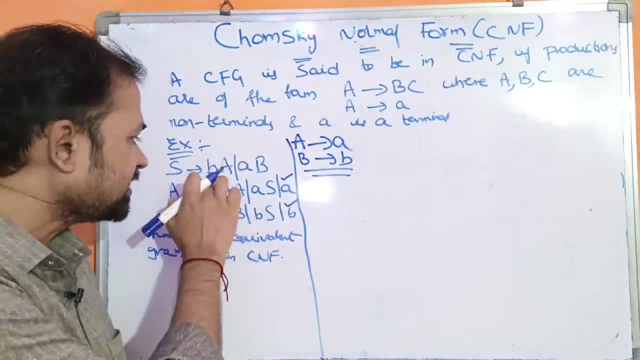 we have to replace each terminal on right hand side with a non-terminal. So what are the terminals on the right hand side? Here B is the terminal, Here A is the terminal, Here B is the terminal. So what are the terminals on the right hand side? Here B is the terminal. 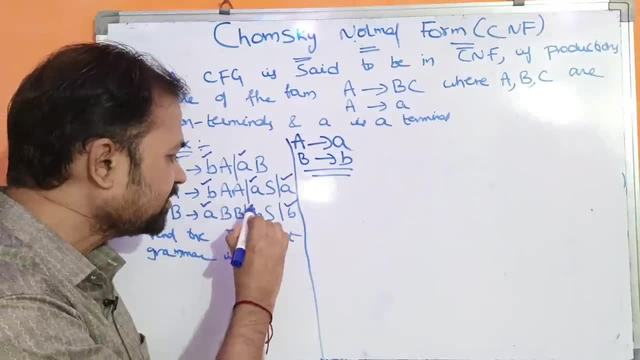 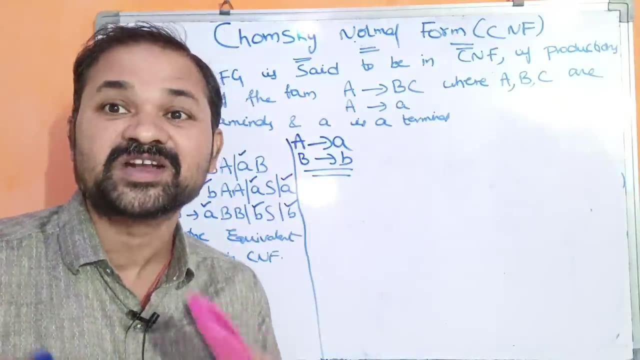 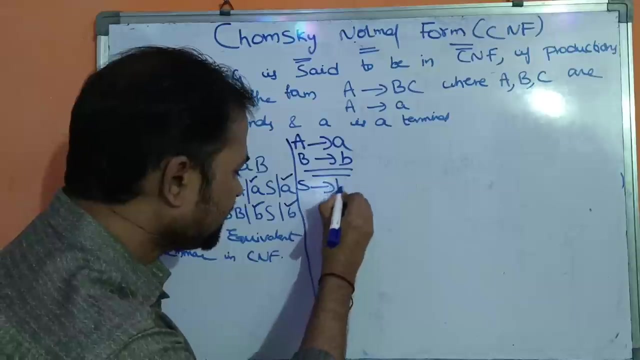 Here A is the terminal, Here A is the terminal, Here B is the terminal. We have to replace all these projections with all these terminal symbols, with non-terminals. Let us see the first projection: S implies B A, S implies B A. So this is the terminal symbol We have. 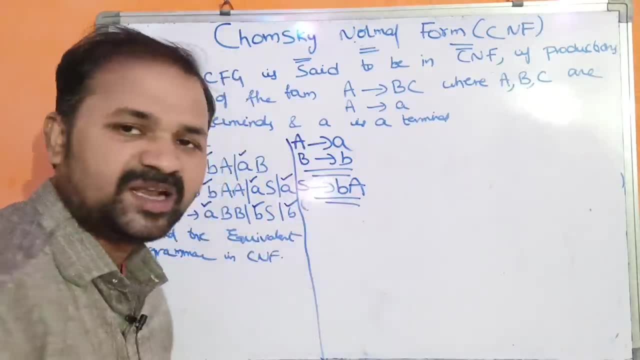 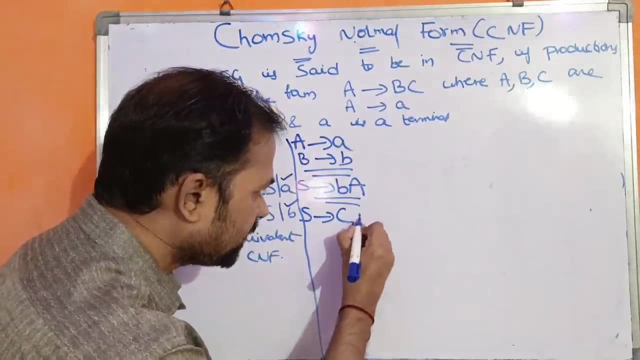 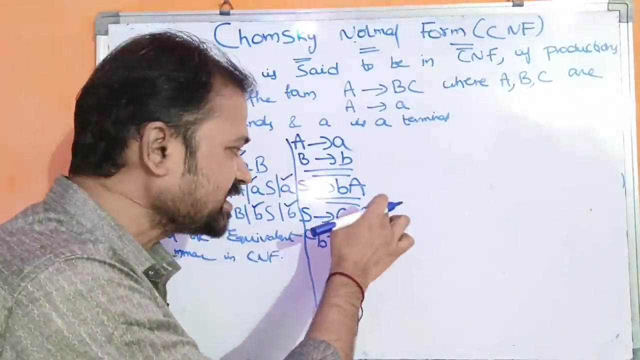 to replace? we have to replace the terminal symbol B with a non-terminal. Let us assume this is C, C, B, A. What is C B here? C B is nothing but B, So we have to replace S implies B, A with these two projections Okay. Next let us consider the second projection, The. 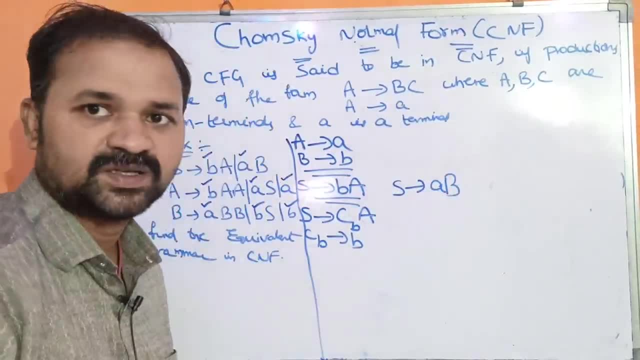 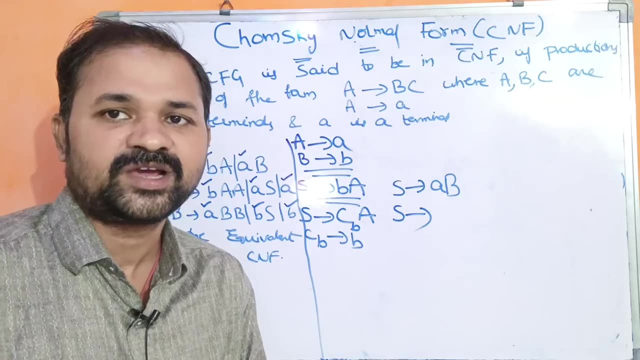 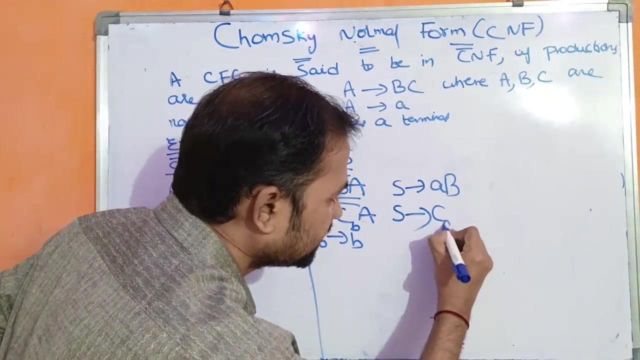 second projection is: S implies A B. So here this is the terminal symbol. We have to replace this terminal symbol with a non-terminal. Okay, So here let us assume that C stands for Chomsky normal form. Here, what is the terminal name? C A In place of C A, we can. 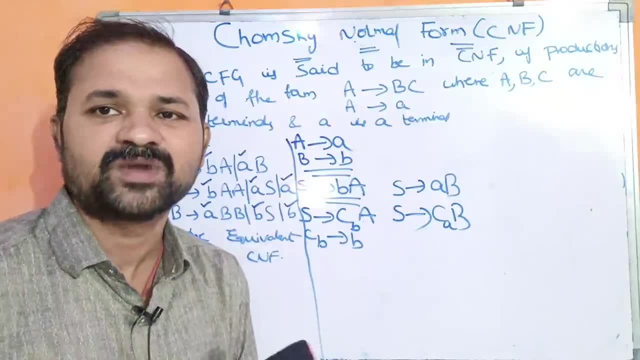 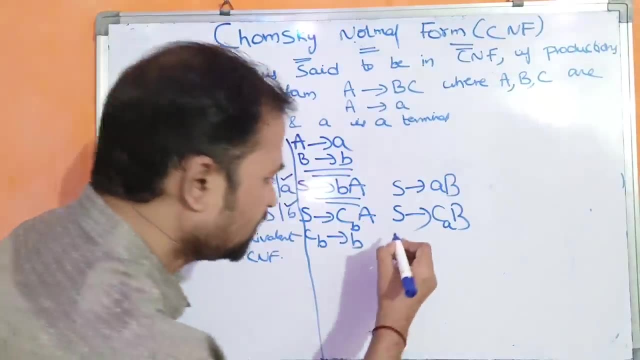 take any other name. It is our choice. We have to give some non-terminal, some uppercase letter: C, 1, C, 2, D, 1, D, 2. It is our choice. A, B, C. It is our choice Where C A implies. 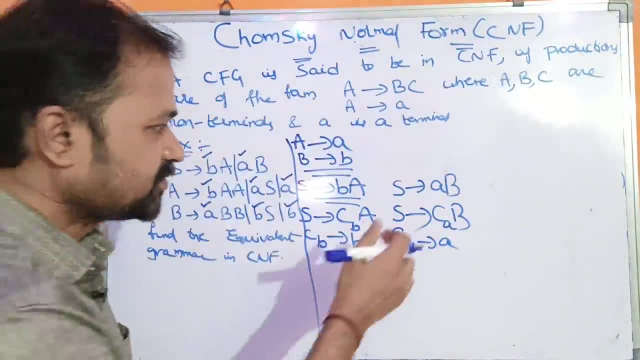 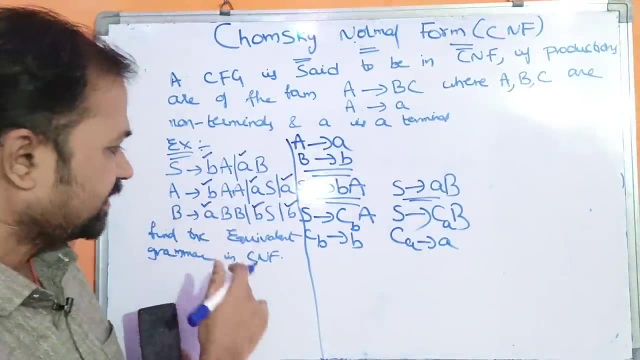 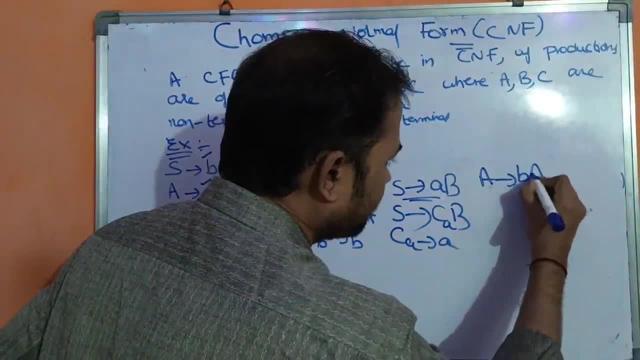 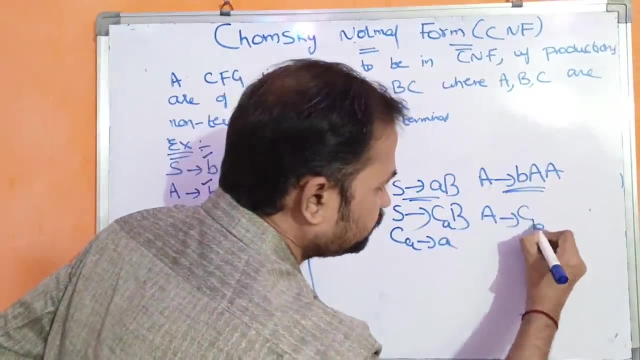 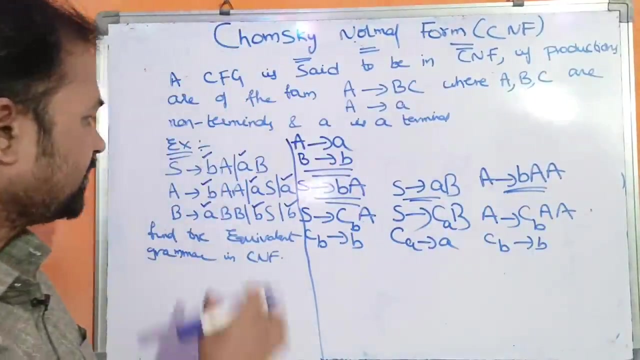 Next one is: A implies B A A, A implies B A A. So replace this B with C, B, A A A. What is C B C? B implies B, C, B implies B. Okay, So next we have A S, A implies A S, So 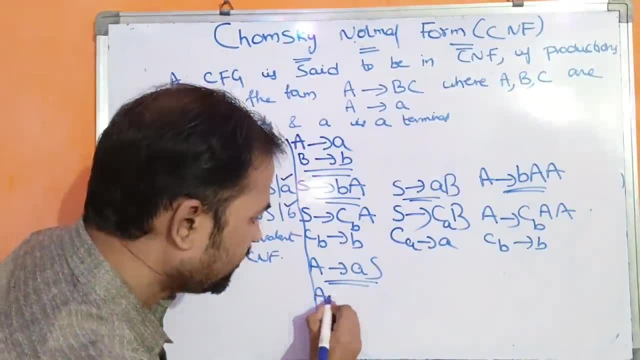 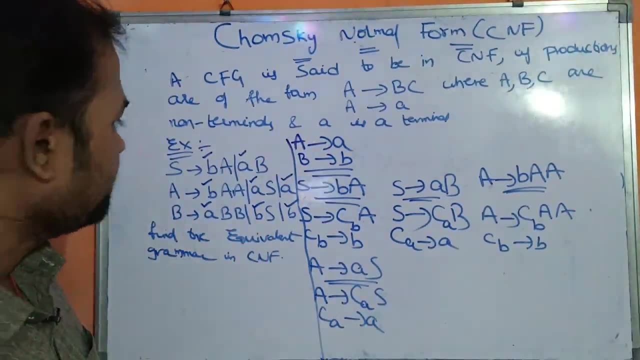 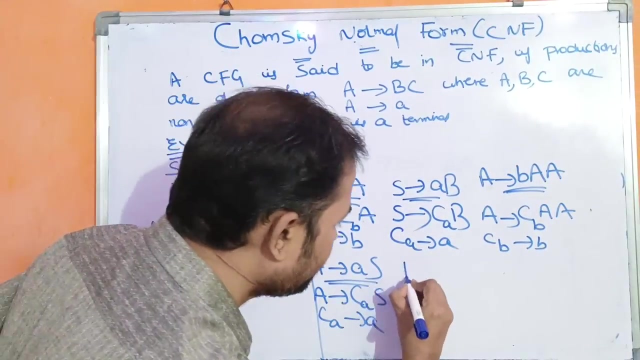 replace this terminal with a non-terminal. Okay, So replace A with C A, C A S, Where C A implies A, So A implies A, A is over. Next A implies A. This projection is already in Chomsky normal form. Next B implies A, B, B, B implies A, B B. So replace this projection. 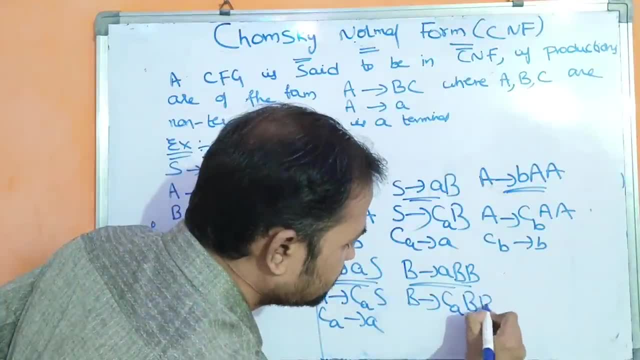 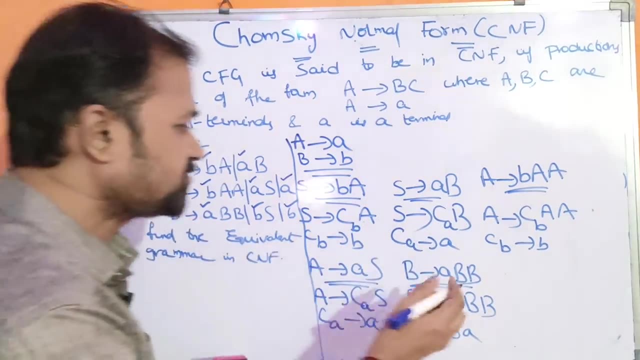 Replace this terminal with a non-terminal: C A, B, B. So what is C A, C? A is nothing but A. So B implies A, B, B is over. Next we have B implies B, S, B implies B, S. So. 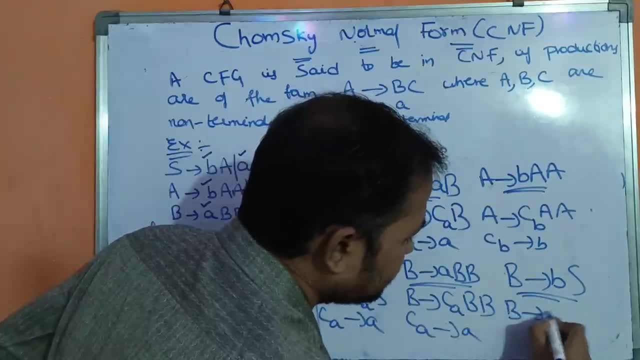 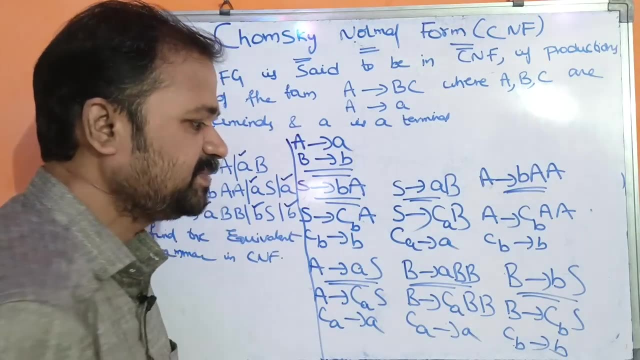 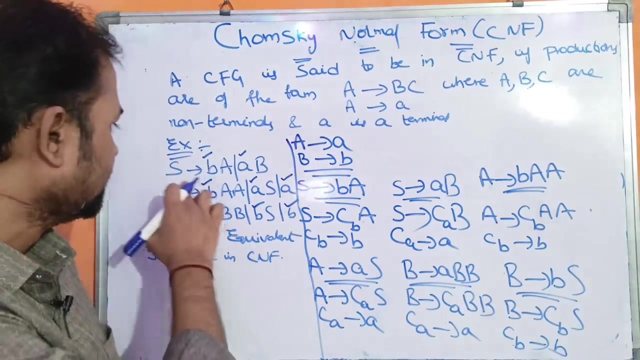 replace small b with C, B, C, B, S, Where C, B is nothing but A. Where C, B is nothing but B, C, B is nothing but B. So here A implies A, B implies B. These two projections are in Chomsky normal form. Next S implies B, A, So this is replaced with these two projections. 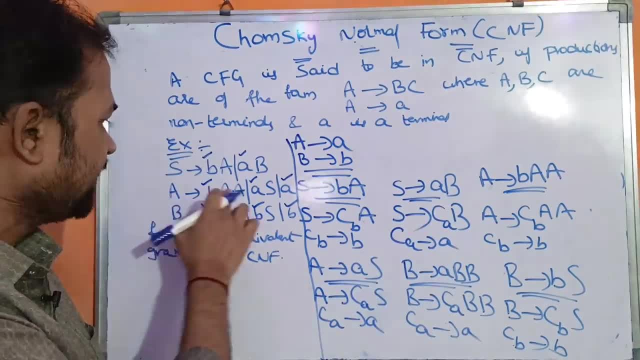 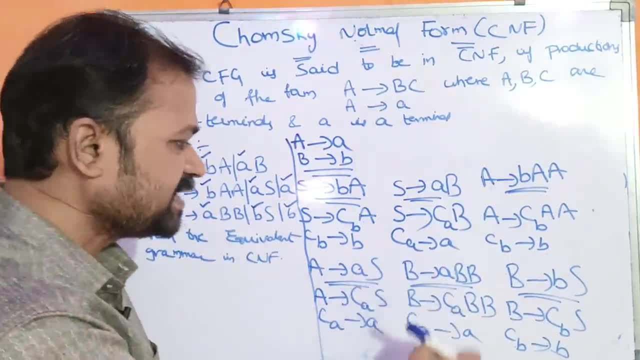 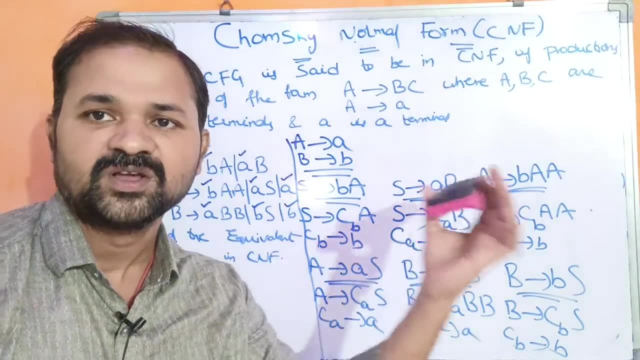 A implies B- A- A Replaced with these two projections. Next, A implies B- A- A Replaced with these two projections. B implies A, B, B Replaced with these two projections. B implies B- S Replaced with these two projections. Now let us observe whether these projections are in CNF or not. 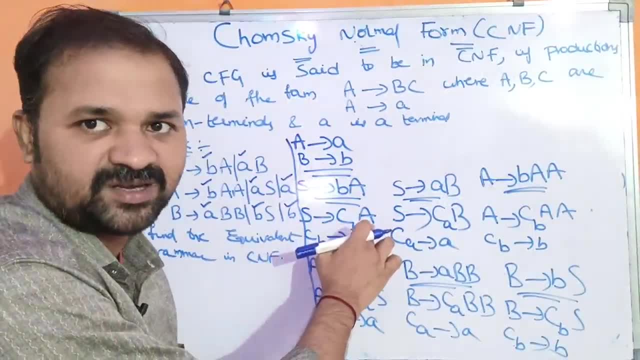 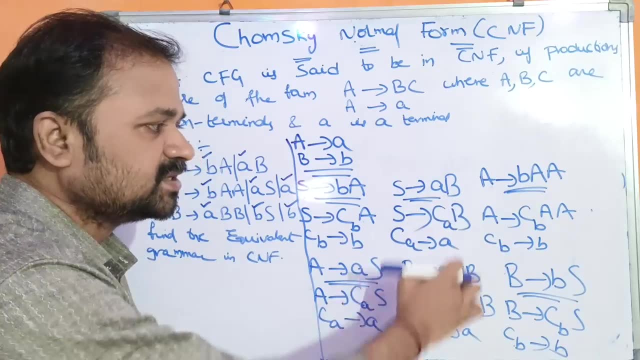 S implies C, B A. C B is non-terminal, A is non-terminal. So this projection is in CNF form. This projection is also in CNF form: C A, B, Two non-terminals. These two projections are in CNF, If you observe. A implies C, B A A. This is not in Chomsky normal form. This. 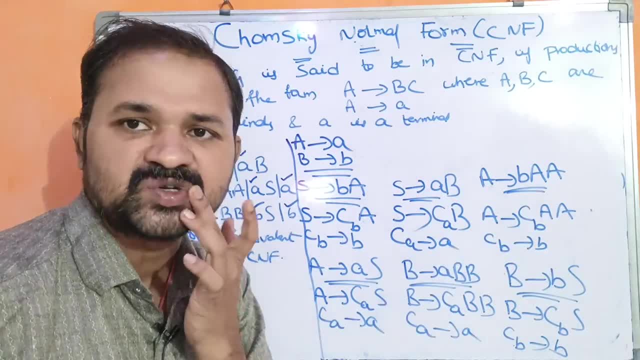 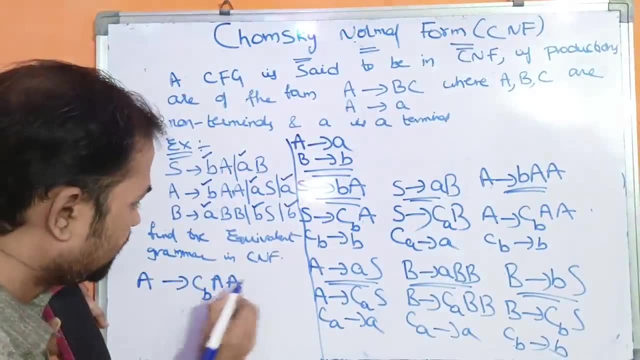 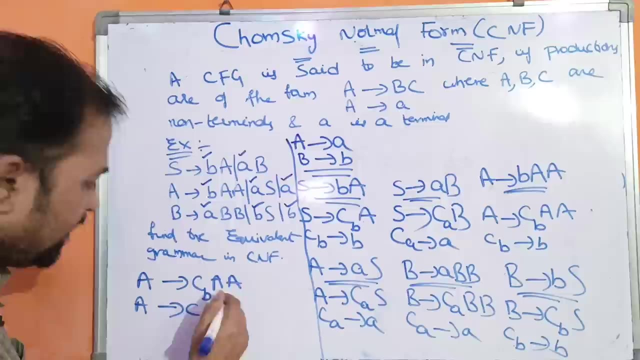 is not in Chomsky normal form. Okay, Chomsky normal form means right hand side should contain only one non-terminal, So let us take A implies C, B, A, A. So this is not in Chomsky normal form. A implies: We know we already have C, B. C B means B, So let us replace this A. 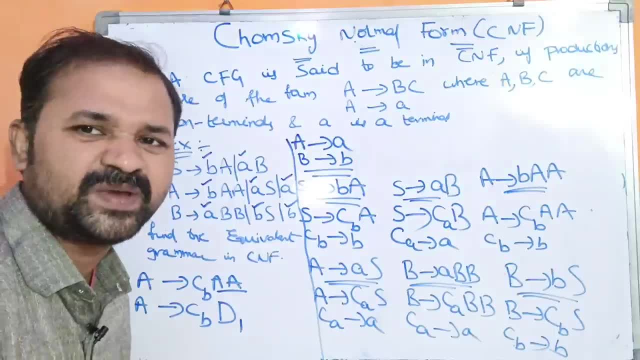 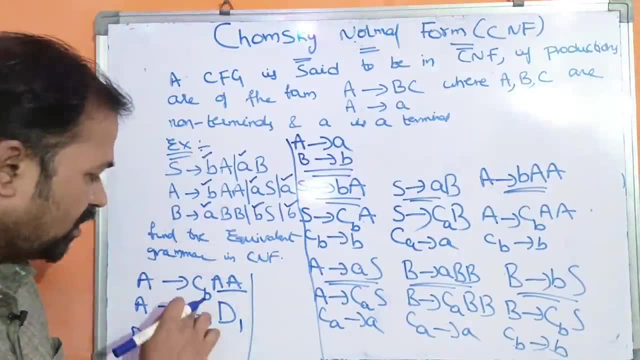 A with D 1.. It is our choice. We can assume any non-terminal Where. what is D 1?? D 1 implies A A, D 1 implies A A, A. So now C, B, D 1.. So we have to replace this projection with these two projections. So we have one. 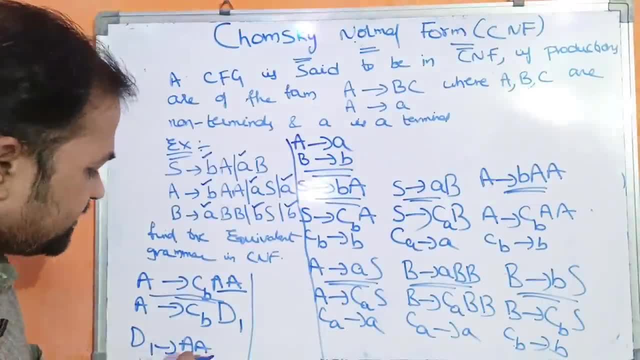 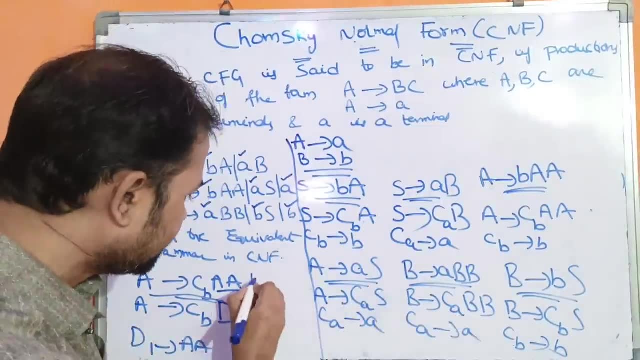 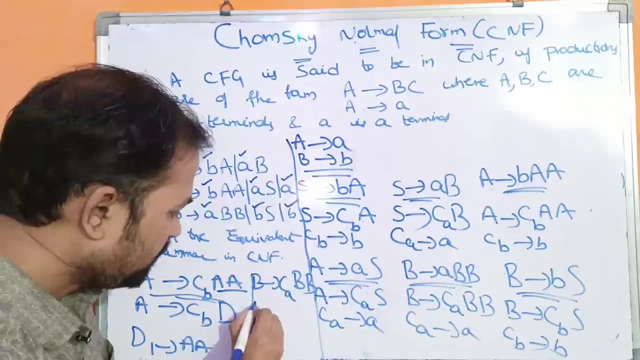 non-terminal. We have another non-terminal: Okay, D. 1 means A, A, Two non-terminals: Okay. Next, the already in Chomsky normal form. Next B implies B implies C, A, B, B, Not in Chomsky normal form. Why? Because we have three non-terminals, So B implies Already. 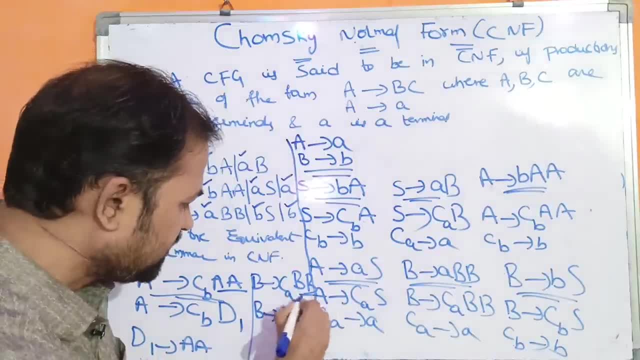 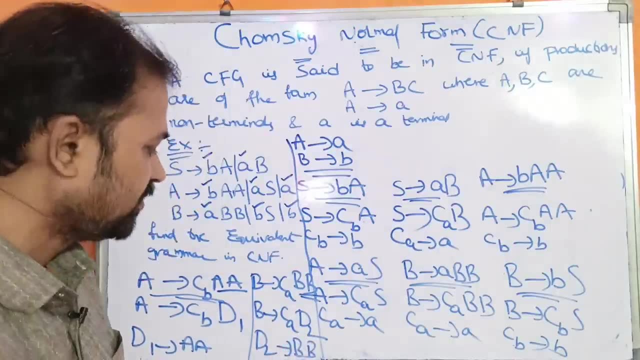 we know C A. What is C A, D A? So replace B B with D 2. D 2. So what is D 2?? D 2 implies B B, D 2 implies B B. Okay, So we have to replace this projection. 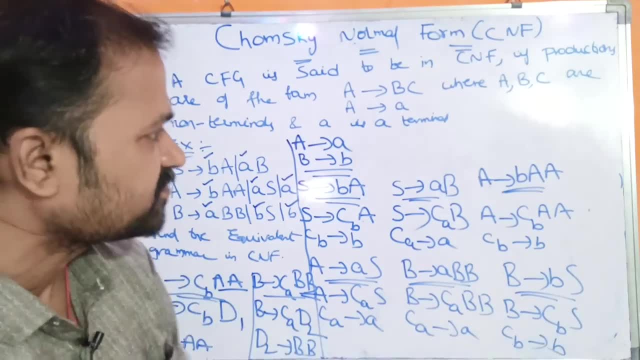 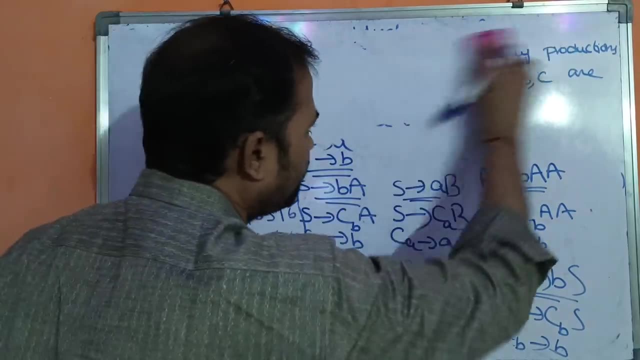 with these two projections. Next, B implies B B, Two non-terminals, One terminal. So this is in Chomsky normal form. So next, So the context-free grammar after converting into Chomsky normal form: The projections are, The projections are. So what is the? 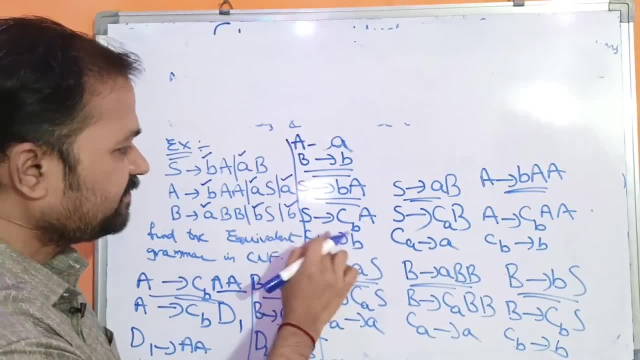 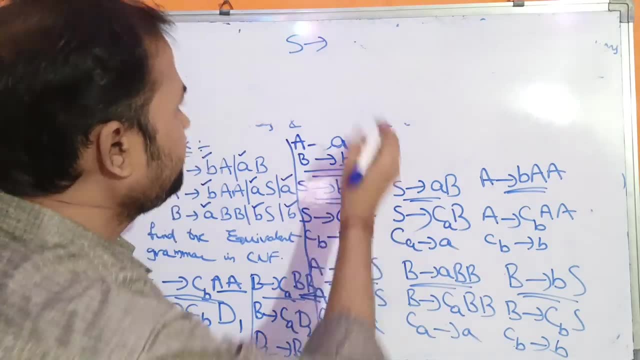 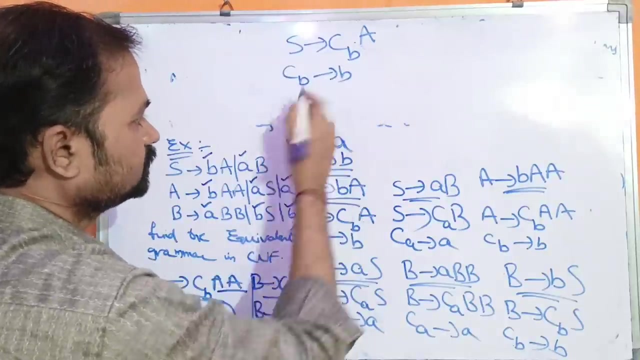 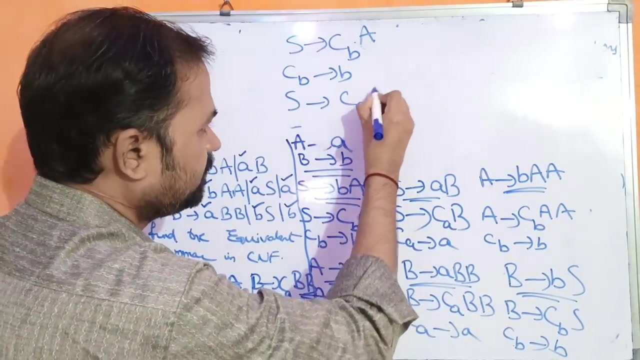 first projection. So we have to replace S implies B, A with what S implies. S implies S implies C, B, A, C, B, A. What is C, B, C, B implies B. Next projection: Replace S implies A, B with S implies C, A, B. Next C A implies What is C A, A. Next A implies. 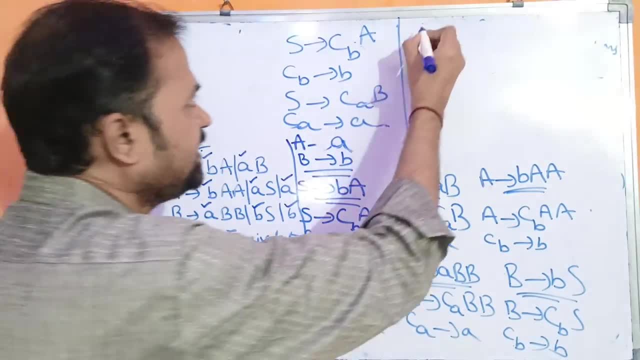 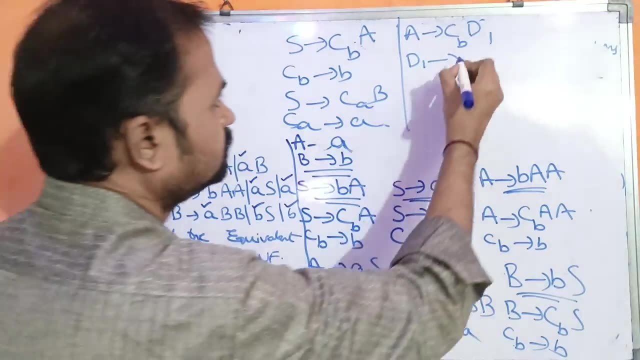 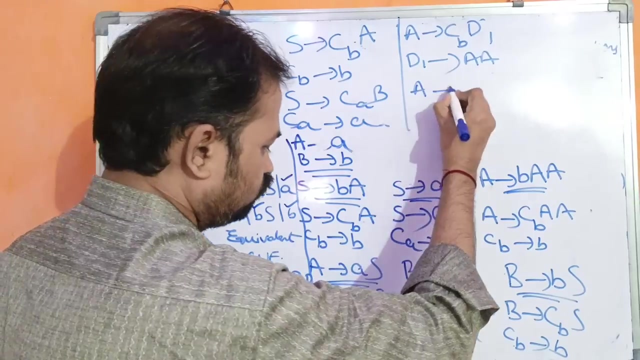 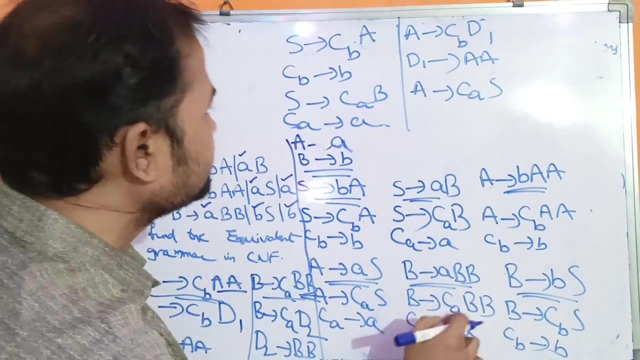 B A. A is replaced with A implies C, B, D 1.. A implies C B, D 1.. What is D 1?? D 1 means A A. Next A implies A A. S is replaced with A implies C A S. C A implies A That is already written. Next one: B implies A B. B is replaced. 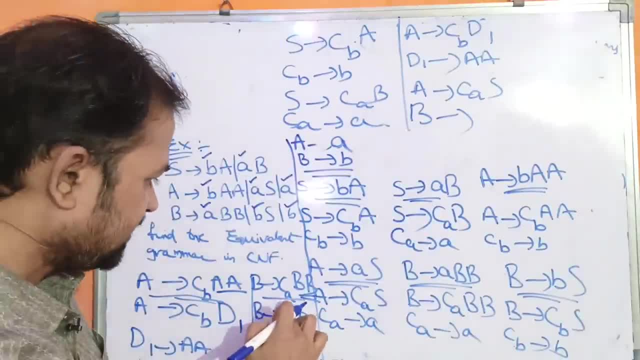 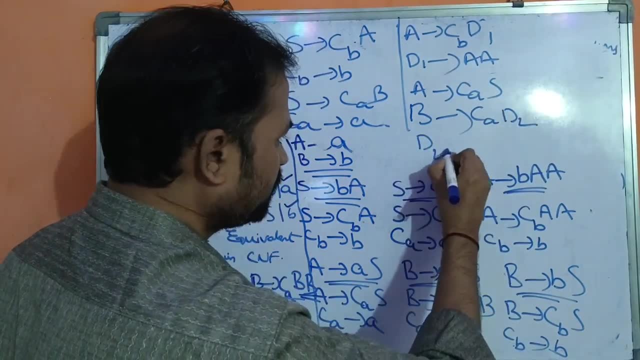 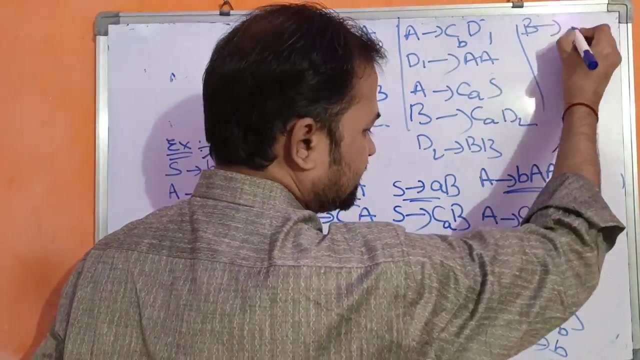 with B implies A, B. B is replaced with what B implies C A, D, 2. B implies C A D, 2. Next B implies B. Where what is D 2?? D 2 means B, B. Next B implies C, B, A. S is replaced with.